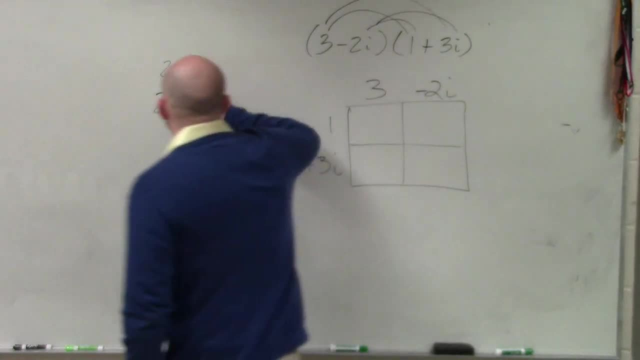 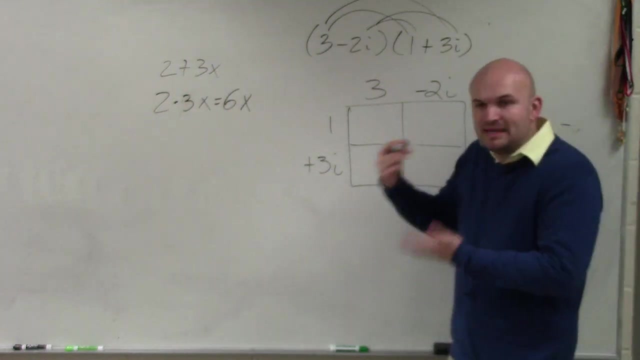 But I can multiply 2 times 3x. That gives me 6x. Well, that's kind of the same thing with real and imaginary numbers. Yeah, we can't add real to imaginary, but we can multiply them. So here is a real times a real. 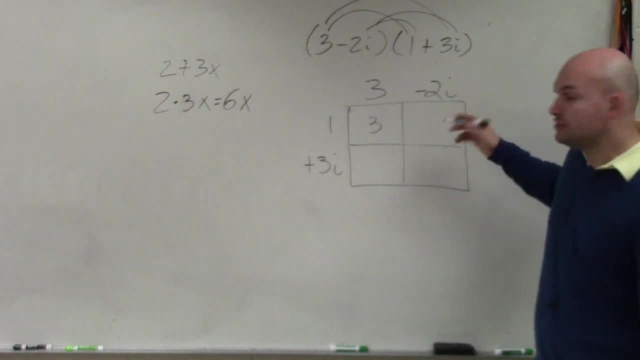 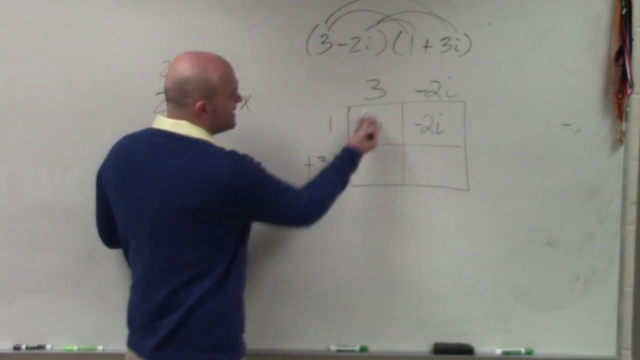 1 times 3 is obviously 3.. 1 times negative 2i, though, is just going to be negative 2i. 3 times 3i again. all you're basically doing when you're multiplying a real times imaginary. 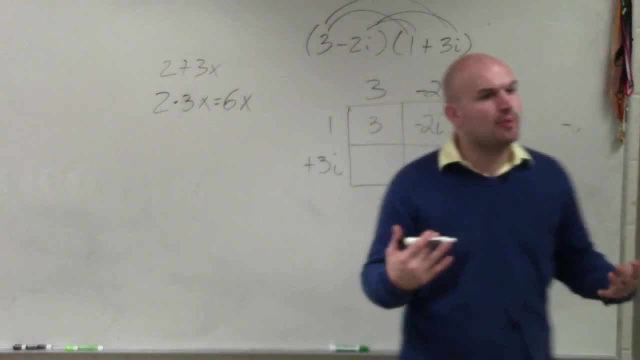 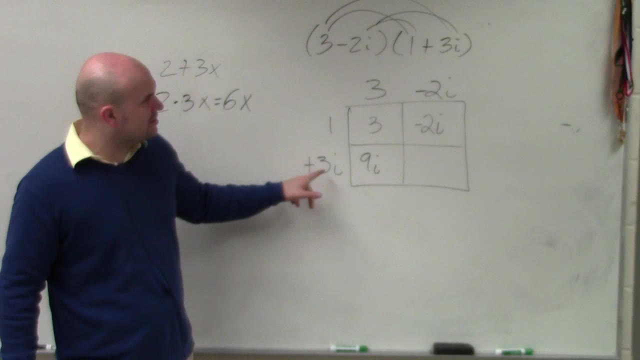 is just multiplying the coefficients, You're just multiplying the real portions of each number. 3 times 3i is 9i. And then over here we have negative 2i times 3i, which becomes negative 6i, squared right. 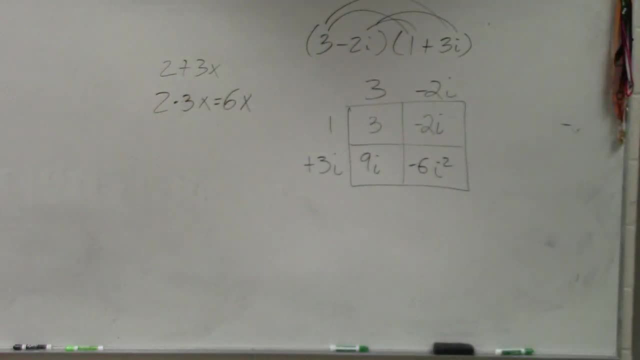 Just like you would have: x times x is x squared. i times i is i squared. Now, remember what I taught I talked about a second ago. Remember what I talked about when we were talking about i, i squared, i cubed, so forth. 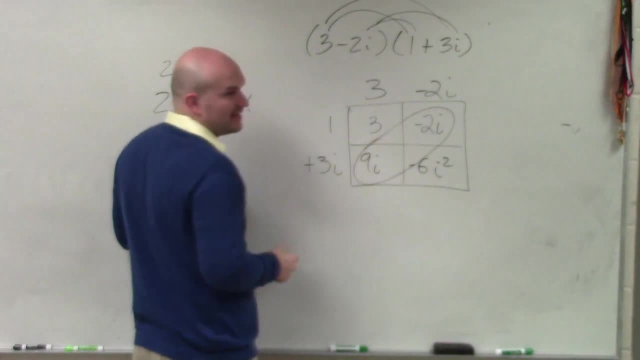 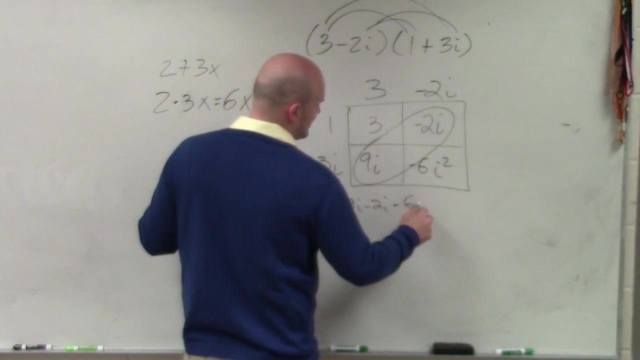 So now we write everything in descending order, We notice we can combine those. So I have 3 plus 9i minus 2i. It should be 7i. I just figured. I'd write it out. This becomes 7i, right. 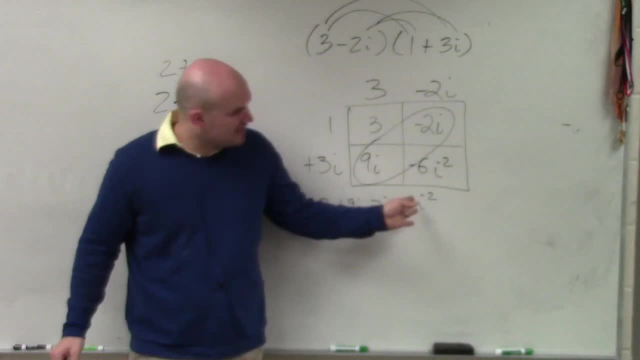 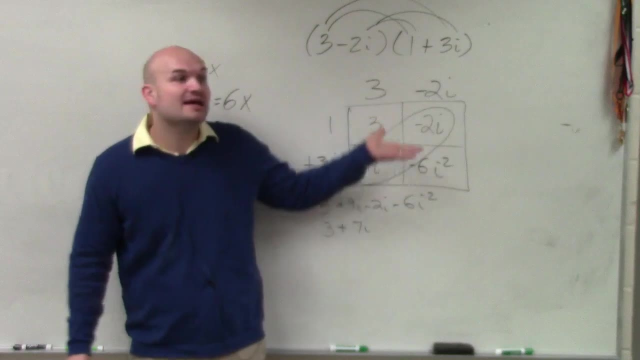 3 plus 7i. Now, ladies and gentlemen, what's i squared represent? What does i squared represent? I don't know. Negative 1.. Minus 6 times negative 1.. Now, what's negative 6 times negative 1?? 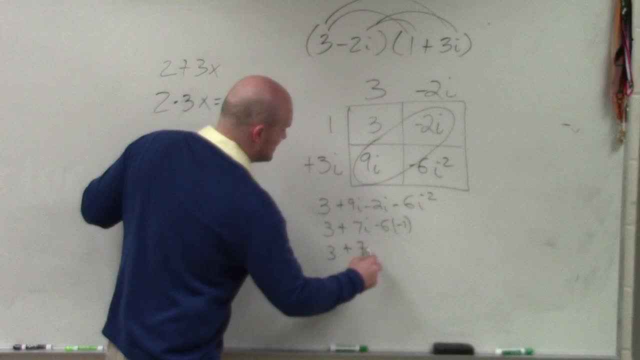 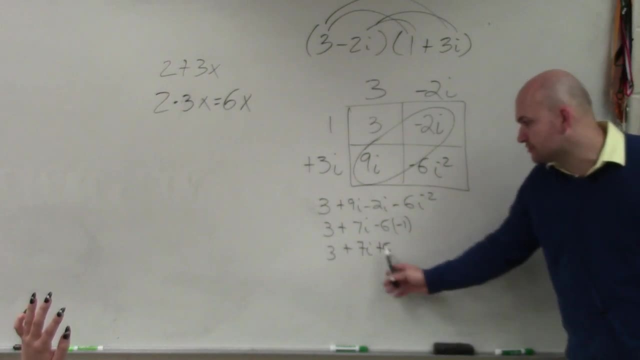 Negative Positive 6.. So I have 3 plus 7i plus 6.. Now I can go back and add my real terms or my real numbers, which is 3 and 6,, which would be 9 plus 7i. 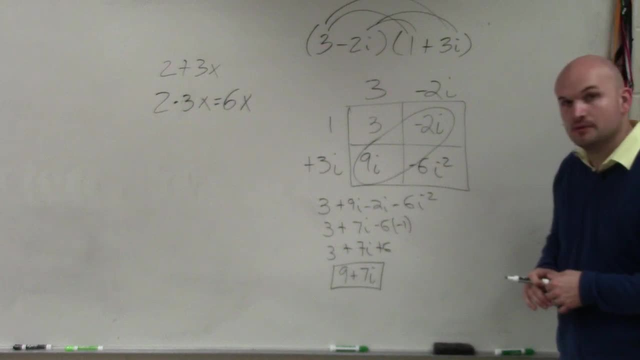 Yes, Why don't you do it in that order? Do what? in what order? Like the equation You like? circle those two. Yeah, you could have just written it like this: 3 plus 7i minus 6 times negative. 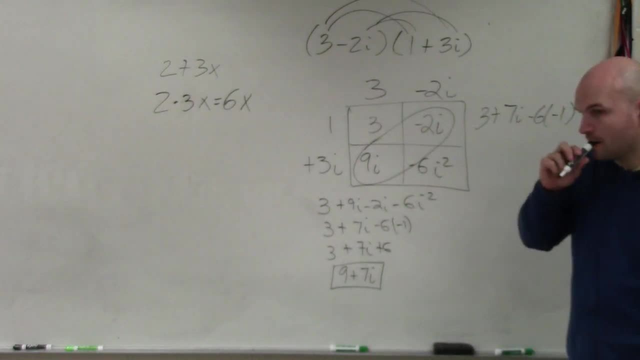 I just did it. I just kind of broke it up one step by step. So just add them what order it is. Oh, no, no, no. The only thing you want to do is make sure at the end you have it in a plus bi format.